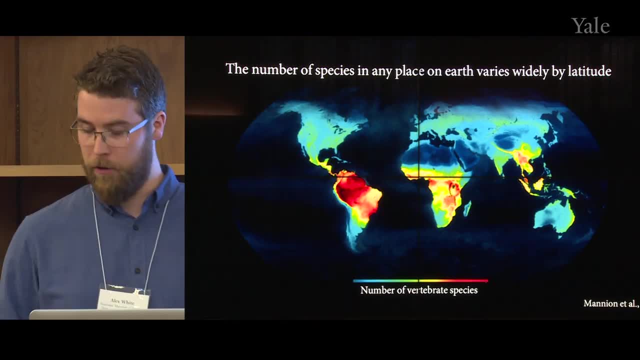 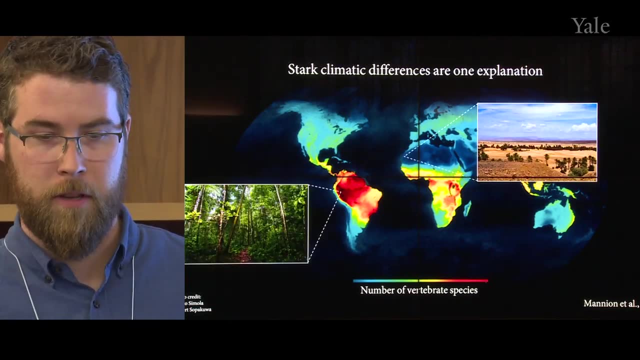 north or south Of the equator. So we see there are many more species in the tropics than there are contained in the temperate environments in North America and Asia. One explanation for those differences is that there are stark climatic differences between locations such 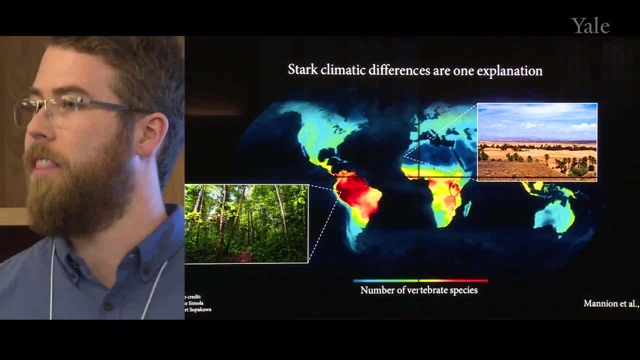 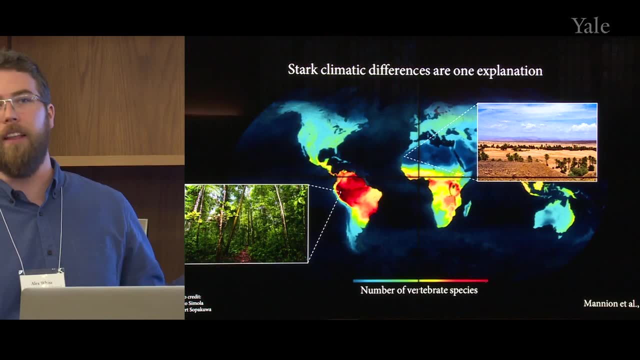 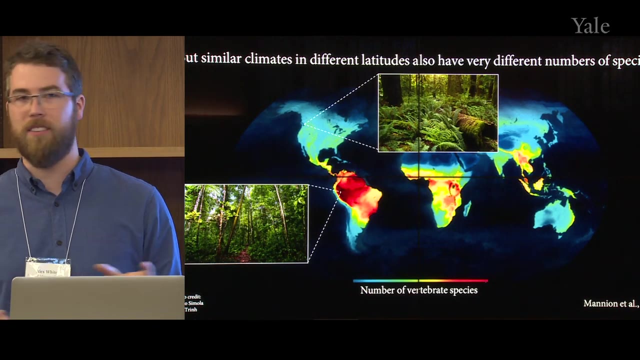 that some locations can afford the many higher numbers of species than are located in others. So this would be just a comparison of, say, the Saharan desert and the tropics of Peru, But there are also locations Where there seems to be much more climatic similarity. This looks like a very lush forest. 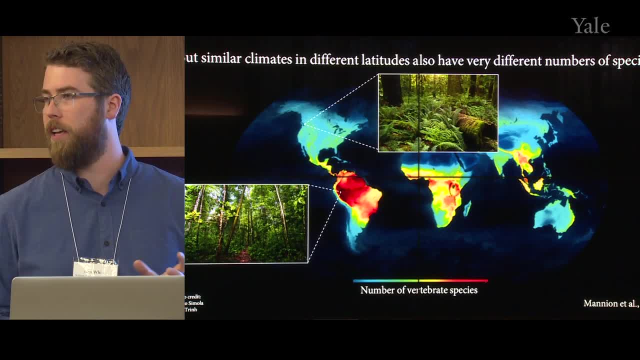 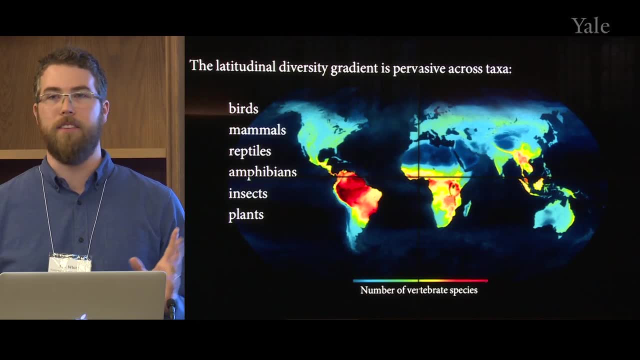 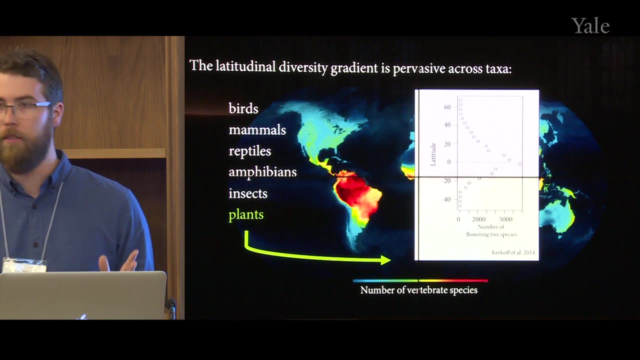 in British Columbia, but there are still many fewer species contained in this forest than there are in Peru. This is a pattern that we see across all taxa. This is not just specific to say, plants or birds. It's across many varied groups of animals And, in particular, 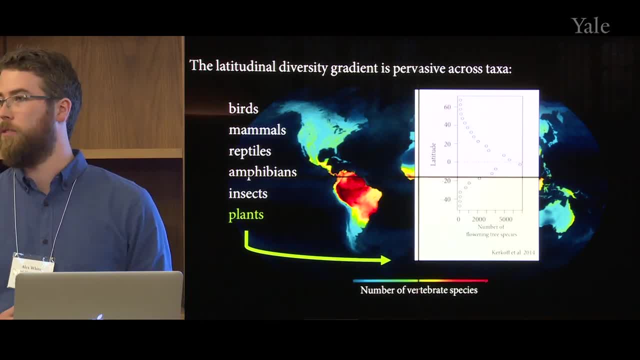 it is true that plants generally follow a latitudinal diversity gradient. So here I'm just showing you the number of flowering tree species on the x-axis And that number kind of binned according to where you are in the earth And you can see on this plot. 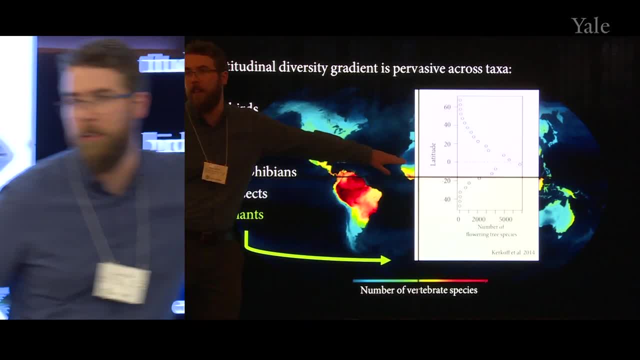 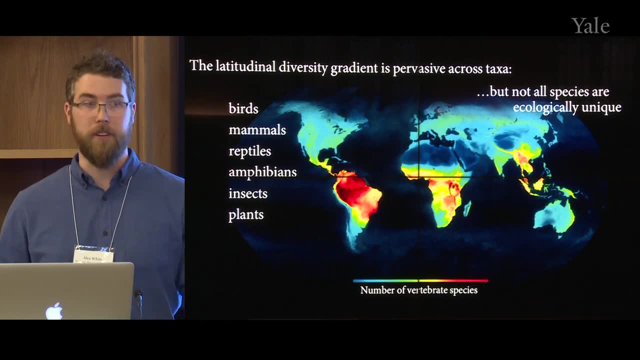 that there are many more species contained in the equatorial latitudes than there are outside of it, But one component. So we have known this pattern for centuries, essentially, And biologists have really been vexed by it And we want to understand why it exists and how it is. 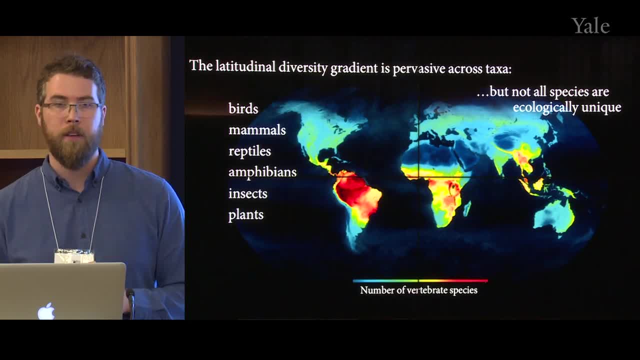 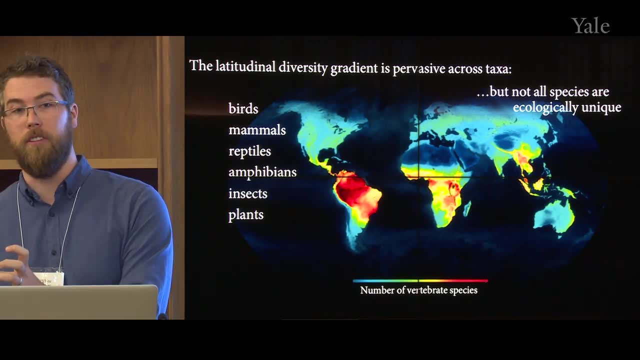 related to other aspects of biodiversity? In fact, I know the answer to this question. It's right here. So the first thing we wanna do is we gotta know who the species are that we're interested in. So not all species are the same as saying there are this number of ecological groupings. 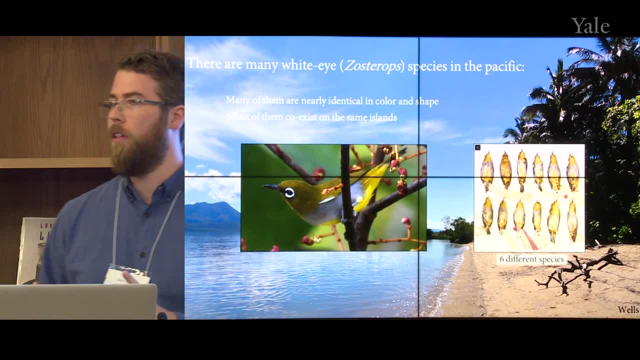 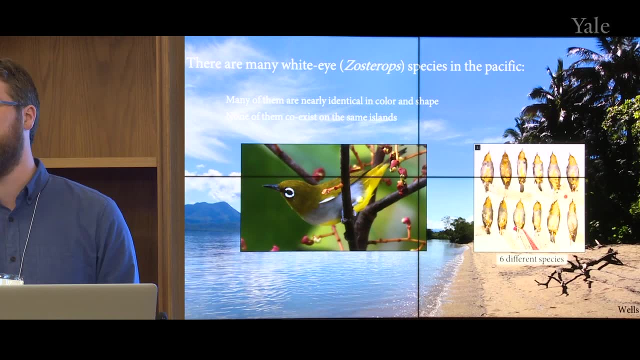 in those locations. So we wanna kind of tease apart the number of species from the number of ecologies. One example of the way that not all species are ecologically unique is an example from birds. The Zosterops genus of birds is a group of white eyes, So this 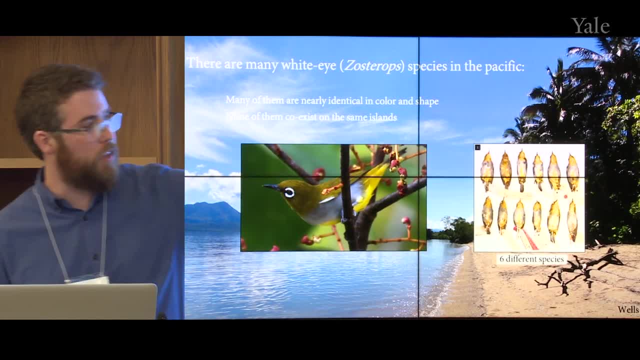 is the white eye here down this side, And the white eye down there is a little red one And the white eye down here is the white eye down here And the white eye down here is image, and the image that I'm showing you on over there is is six different. 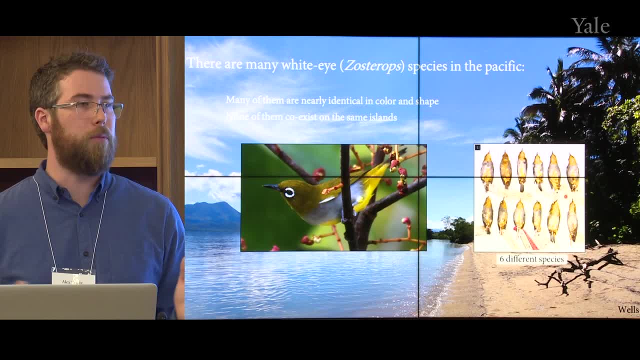 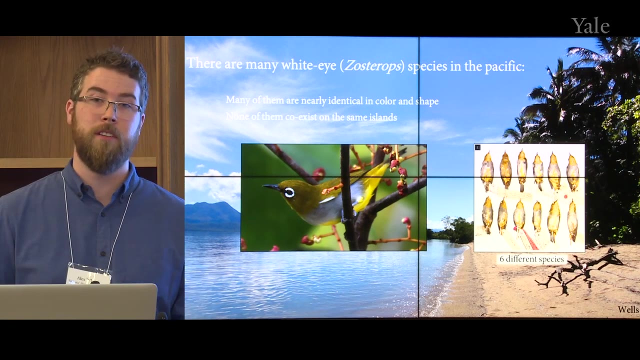 species of white eyes, and so to you know, the lay observer, it might just look all like the same bird, right? so what what's true is that it's just because there are six different species. really we could call these kind of the same ecology: there's six species, but maybe one ecological function, and so we want to. 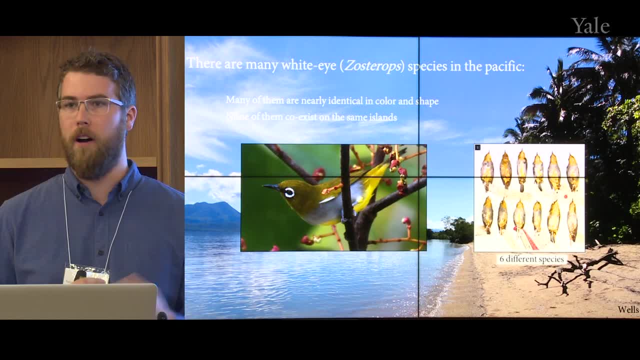 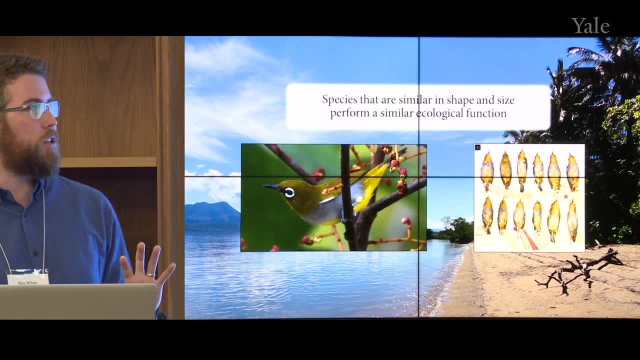 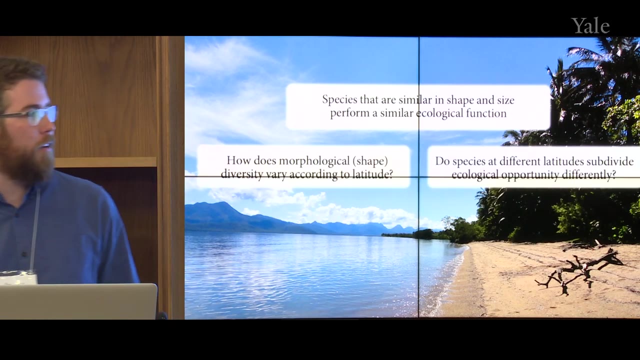 tease apart these aspects of, say, shape from the other taxonomic diversity that we described in museums for centuries. so we know that species that are similar in shape and size perform a similar ecological function, which raises two questions. the first is: how does shape diversity vary according to latitude we 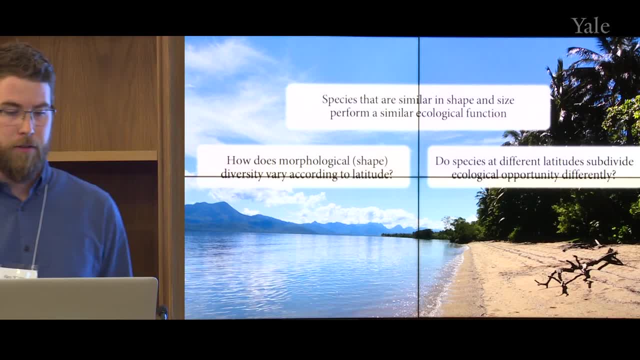 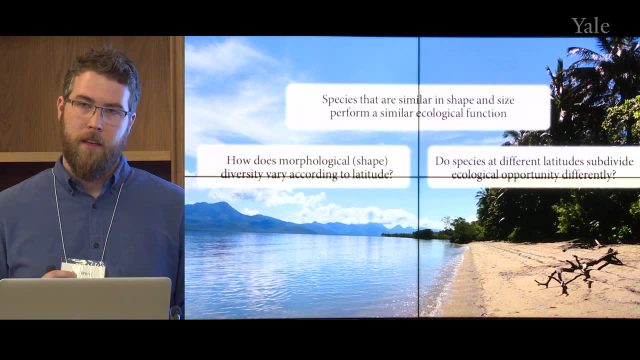 know that the number of species changes according to latitude, and that informs another kind of deeper fundamental question is: how does shape diversity vary according to latitude? and that informs another kind of deeper fundamental question about evolutionary biology, which is whether species at different latitudes have some sort of different ability to carve up the ecological space in those places. so 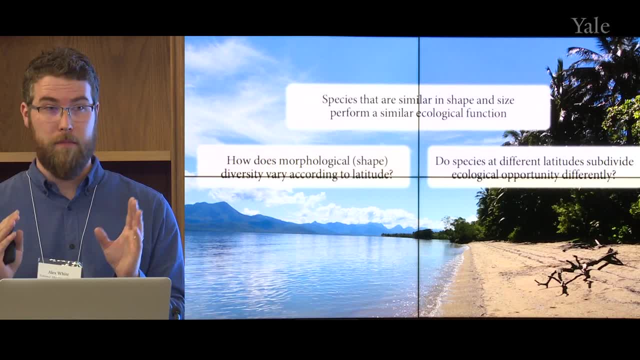 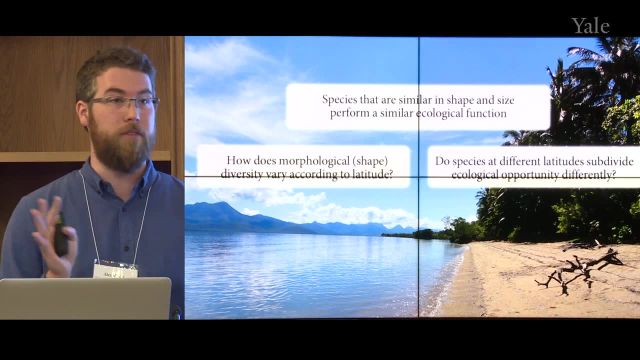 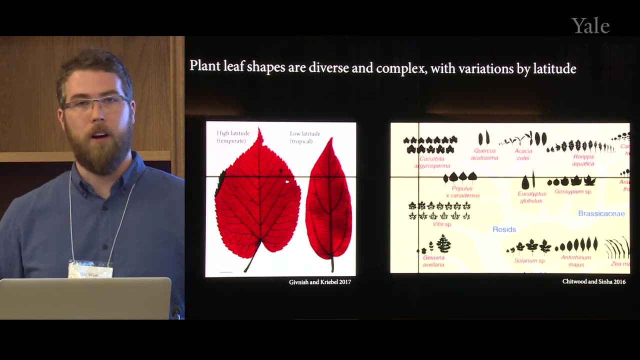 is it that tropical species are really just able to become more finely and specifically adapted towards one ecological function, and that's the reason why we've jammed so many more species in those locations than otherwise. so plant leaf shapes are obviously very diverse and complex. we've certainly all walked around in a 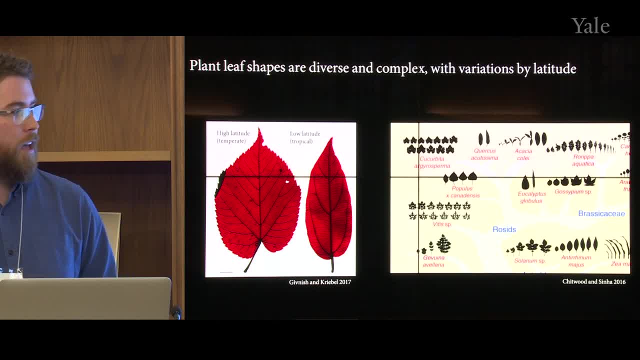 forest and looked around and seen many different shapes and sizes. there's just a schematic there of some of the different shapes of leaves as they're in particular species as they develop. so there's obviously also changes according to development, but there's also this very basic pattern that's known in plant. 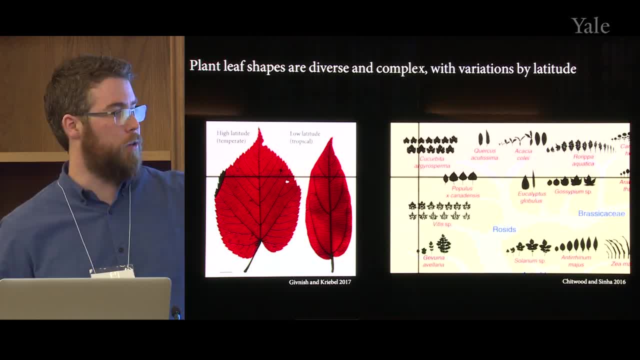 shape according to latitude, which is that high latitude, temperate locations have more toothed leaves than those that are in the middle of the forest, so that's why we're calling them toothed leaves. so the edges of this leaf are called toothed, and this tropical leaf has what's called an entire margin, and so the absence of 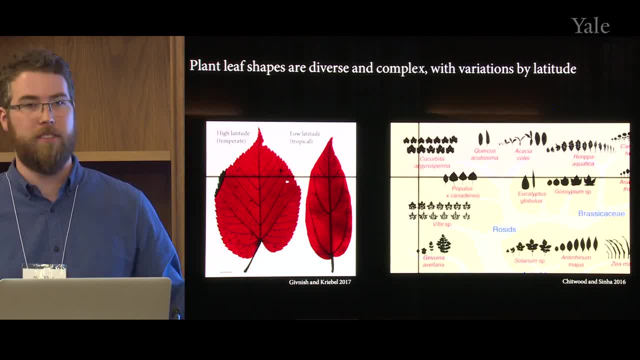 toothed in tropical locations. so evolutionary biologists have been trying to study this difference, and we're kind of interested in a next level of complexity, one that doesn't necessarily involve just saying this is tooth, this is not, but something more complex. so we've heard a lot this morning about the 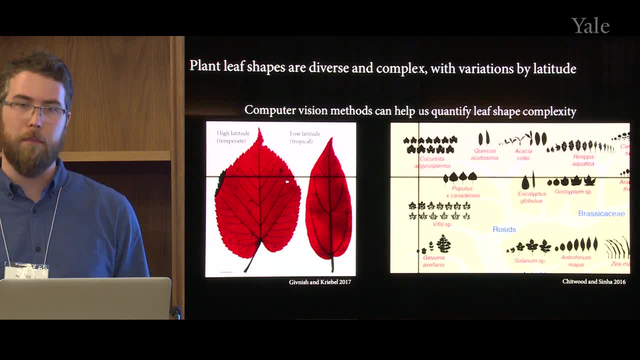 kind of magic of computer vision and how to determine which leaves are more complex and which are more complex than others. and so we've kind of taken a look at the kind of magic of computer vision and how we're trying to determine which is the. it might help us reduce some of this complexity to understand shape differences. 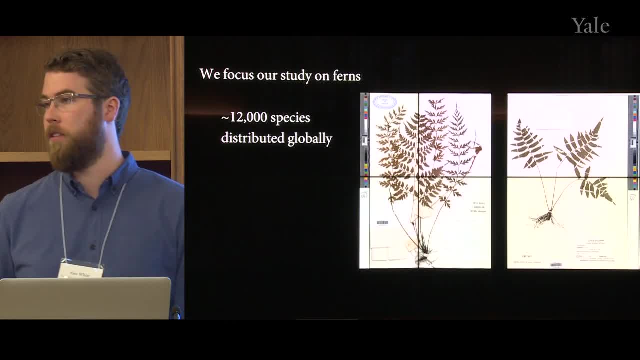 So we focused our study on ferns of the world. There are about 12,000 species of ferns distributed globally. Here are two such examples, two specimens that are contained in the US National Herbarium, and they're two different species. 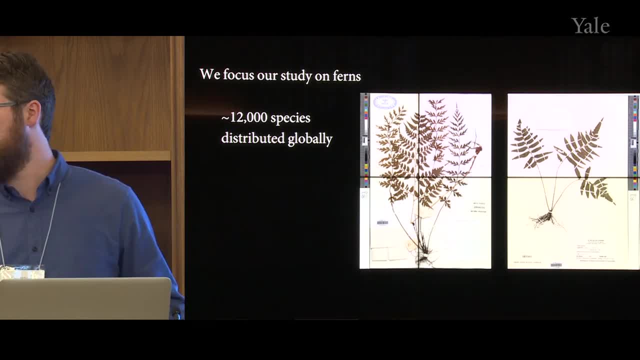 I think it's fairly obvious that they look very different and that difference is very complex. So it might be difficult to measure the difference between those two organisms, except for if we might use something like a convolutional neural net to extract that information. 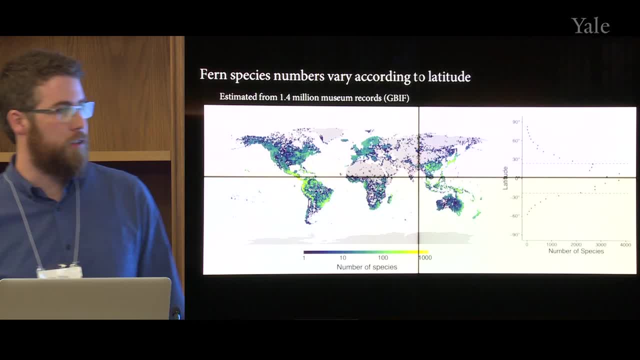 The distribution of ferns of the world follows a similar pattern to what we find among other organisms. There are many more species contained in the tropics. This is actually just a quick estimate of the number. There are a number of species that might be located in different places on Earth. 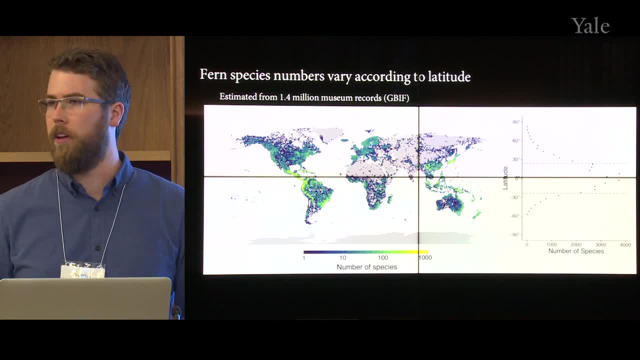 using a data set that we heard about this morning called GBIF or the Global Biodiversity Information Facility. So I took all of the occurrences that existed on GBIF for ferns and mapped them according to where they were found. These are for all occurrences that had some decimal lat and long. 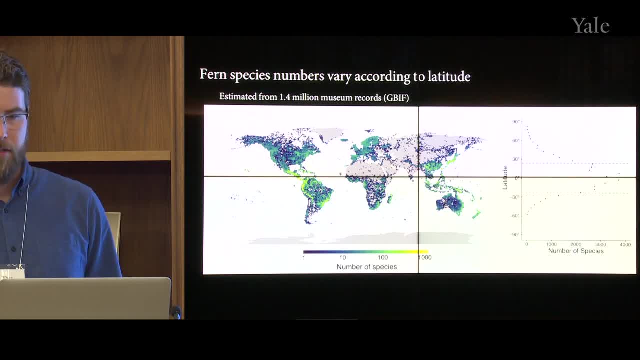 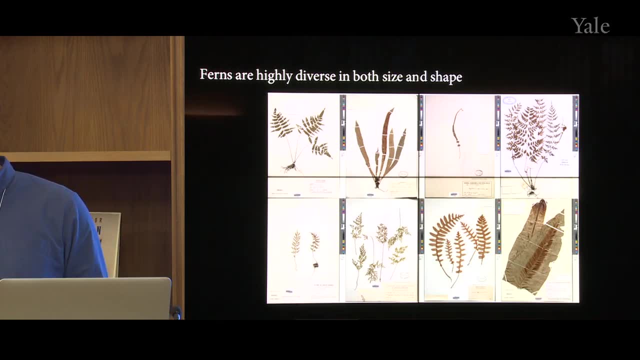 We find that, again, there are many more species contained in the tropics. Ferns are also highly diverse In both size and shape. So here are eight specimens of eight different species. We can see that there's really a lot of complexity here that we'd like to understand. 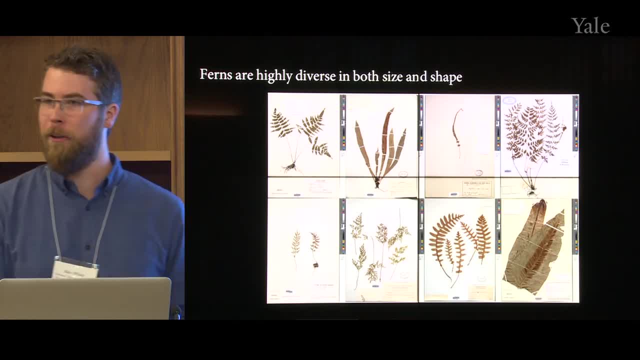 but it's not so obvious how we might get to that answer if not for some large-scale kind of method that would help us kind of put all these eight species in some sort of high-dimensional or low-dimensional space based on their differences, which are clearly very high-dimensional. 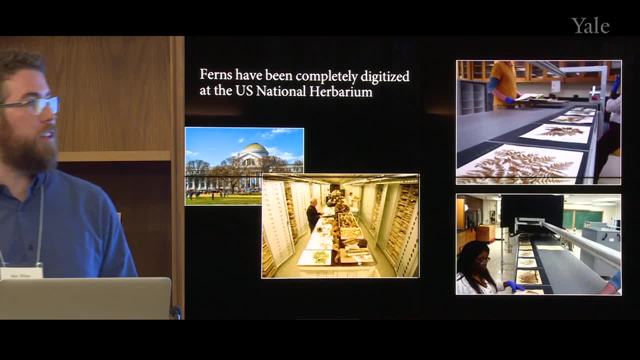 So ferns have been completely digitized at the US National Herbarium. We heard about the digitization effort this morning. I just want to show you this is kind of what an herbarium looks like. It looks almost nothing like that normally. 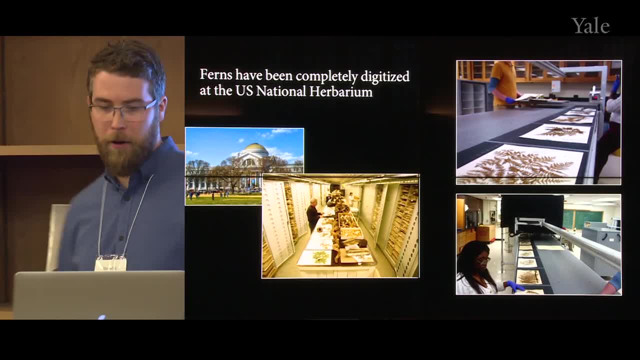 That is just when you want to get a really cool image for everyone to look at. Normally it's just a bunch of file cabinets that are closed, But they're flat specimens that we can then digitize, which is a really useful way in which we've kind of moved forward. 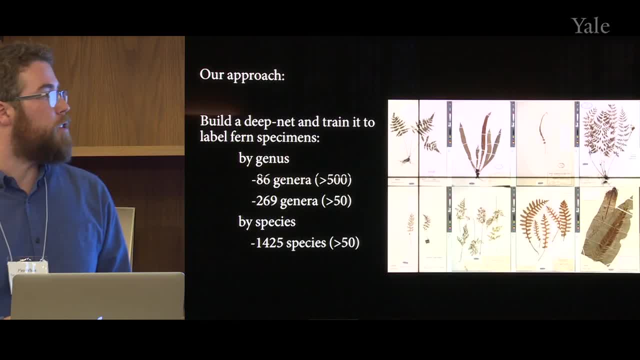 with this project. So our approach was to take all of the specimens that are contained, all the digitized specimens that we could find for ferns, not only in the Smithsonian but also on a larger kind of international collaboration, mostly focused on North America, called the Integrated Digitized Bio Collections or iDigBio. 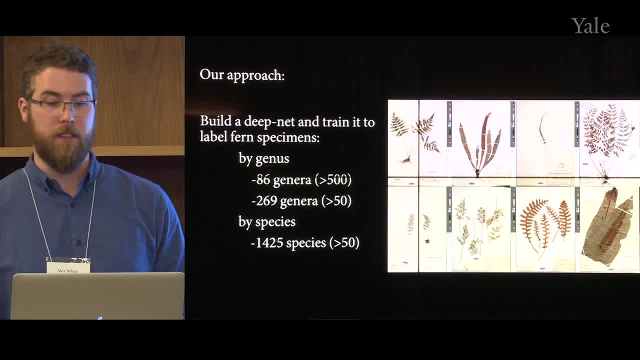 So we took images from iDigBio as well as images from the Smithsonian to train three models. The first model was to identify or label the specimen according to the genus of the plant, of the fern on the image, And we only we built kind of. this is our simplest model, which is that we took genera that had at least 500 occurrences in our data set. 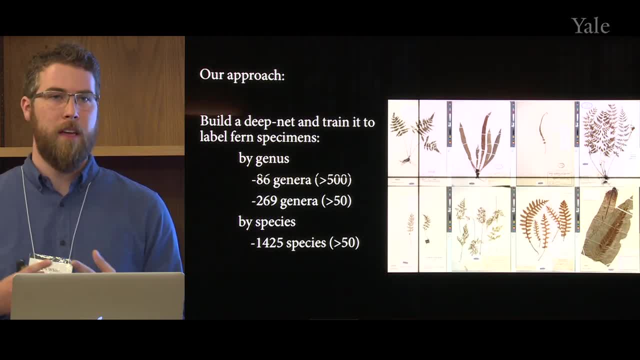 So we've kind of alluded to it all day. but it's more difficult to learn features when you have fewer training examples. In this case, we're going to show you how to do that. So we've kind of alluded to it all day. but it's more difficult to learn features when you have fewer training examples. In this case, we're going to show you how to do that. 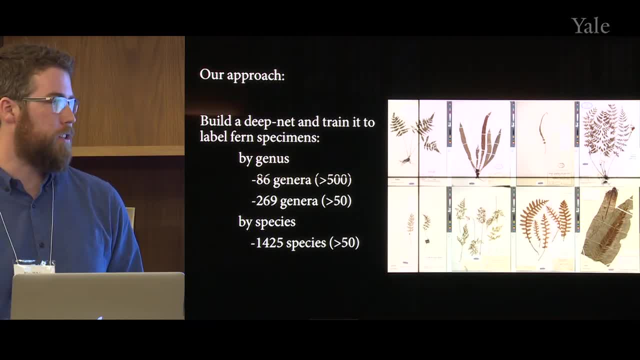 In this case. we're going to show you how to do that. In this case, we wanted there to be at least 500 training examples for each genus, But we started to change that up as we found that our original model was incredibly accurate. so we wanted to kind of test the limits of it. 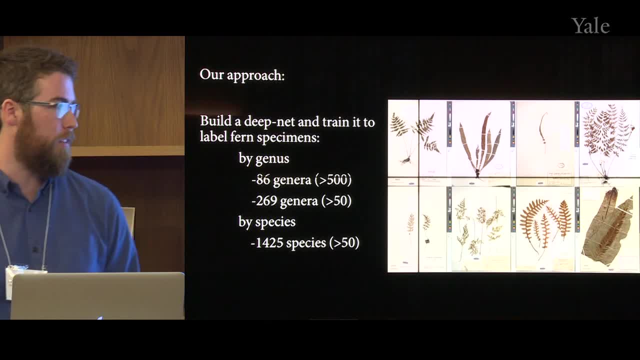 But we started to change that up as we found that our original model was incredibly accurate, so we wanted to kind of test the limits of it. We made a model where there were 50 specimens per genus. So a lot of this is related to where botanists have collected plants around the world and how those collections have been built. So there's somewhat of that bias in terms of you know where the specimens are distributed and which specimens we've found, But partly rare specimens tend to come from places that botanists don't visit very often and might be unique. So that's kind of why we kind of moved around like this. 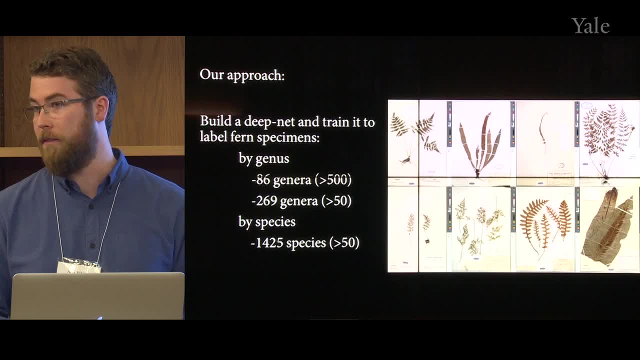 So we built a genera model with 269 genera for about 50 specimens And then ultimately a 1425 species model with at least 50 specimens per species. So in each case the model gets more complex and it will be more challenging for our model to distinguish. 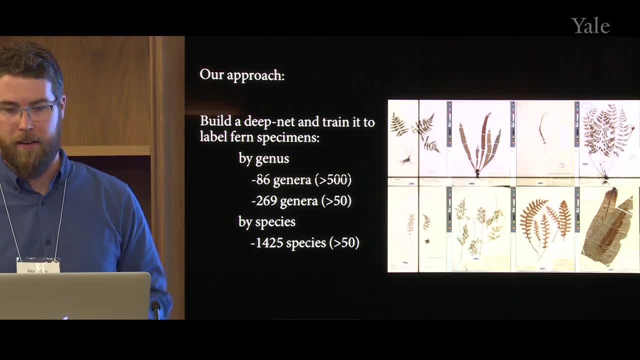 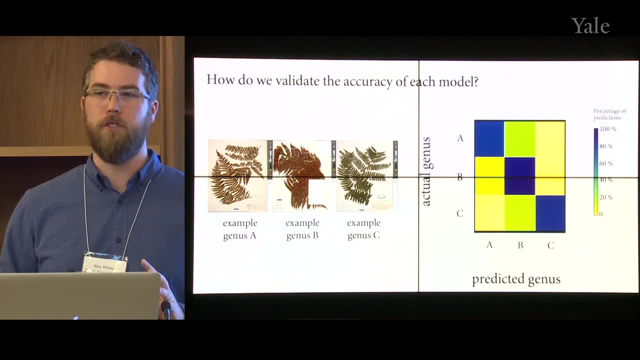 between the different labels that we're going to give it. So we talked a little bit this morning about confusion matrices, But this is essentially how we validate the model after we've trained it. In the first case, we had hundreds of thousands of images and we carved up our training set into 80% of those images that we would train our data with. 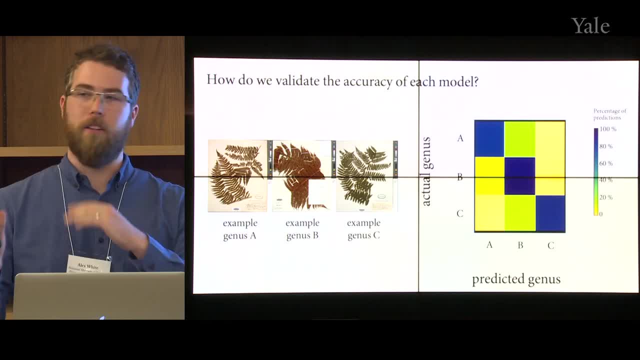 And 20% of those images which it had never seen. we're now going to ask: How good is this? How good is it at giving the correct label that we actually already know? So for a given genus, the actual genus A, we have some proportion of the labels that the neural net then generates for that genus. 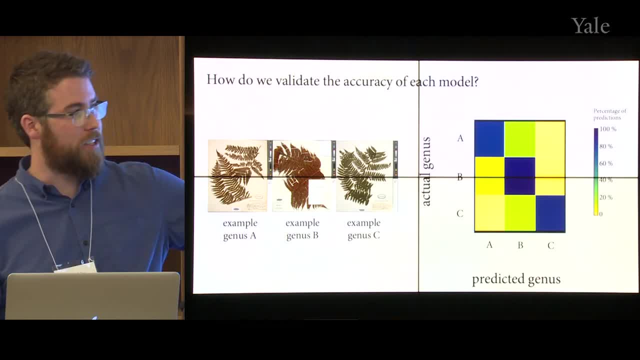 And we can plot those accordingly in that A row. What you want to see is that blue diagonal where it would be 100% of the actual genus was predicted to be A at the bottom, But sometimes there is some confusion. It's true that the model is certainly not perfect. 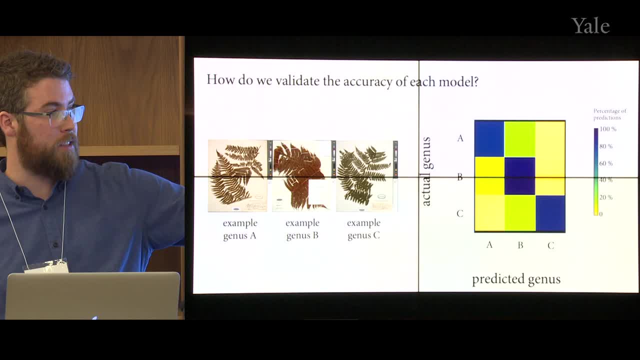 And oftentimes that confusion happens between things that are closely related. So in this case we're looking at three genus from a family of what's called the tree ferns, And there tended to be more confusion, say, within this family than outside of it. 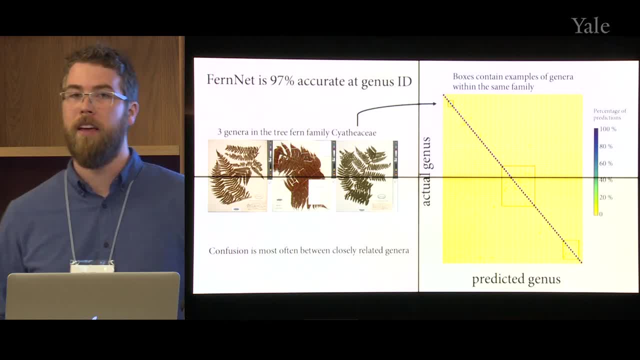 But the model was incredibly accurate overall. It had 97% accuracy to identify the genus In our 86 genus model And that accuracy didn't change too much when we moved to the 269 genus model And you can see that it was highly accurate across that diagonal. 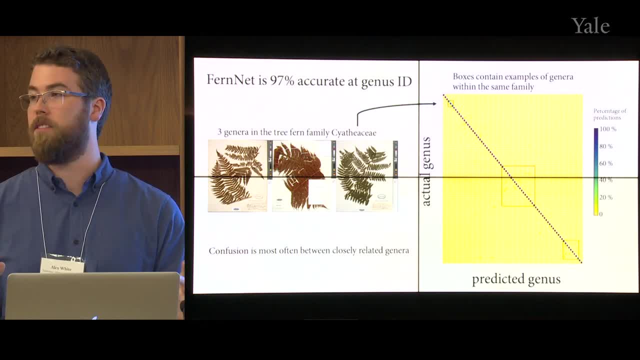 But it's those boxes that contain families of genera where you see more confusion. So that's telling us that the model is operating according to the biologist's intuition. It's not accidentally making mistakes too widely outside of the exact type of mistakes that a less trained body would make. 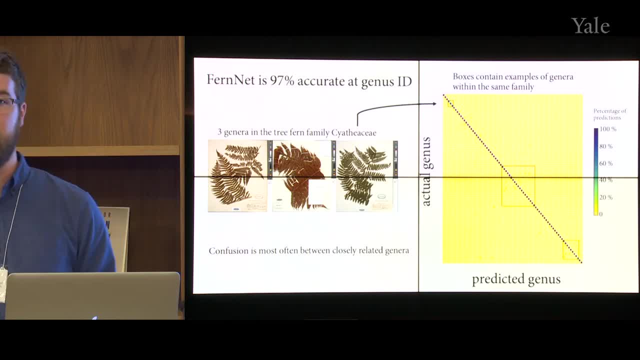 If they were making identifications in the field or if they weren't using a hand lens. Many of these genera are distinguished by traits that are essentially not visible by the human eye, So it's pretty incredible, in that way, that the machine is actually learning patterns of differences that we don't currently use to differentiate between them. 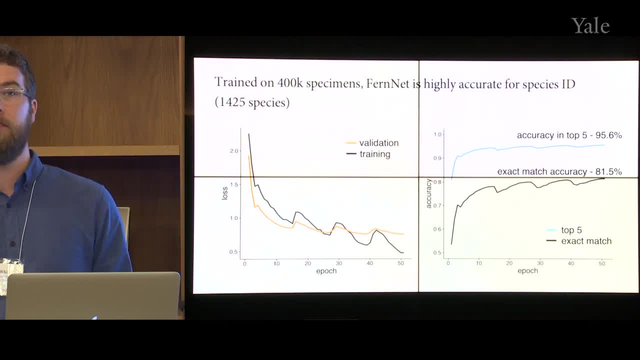 So when we trained our model on species, It remained a highly accurate model And some of the inaccuracies were, I think, forgivable. First off, I just am showing you two plots. These are kind of basic metrics that you gather as you train a neural network. 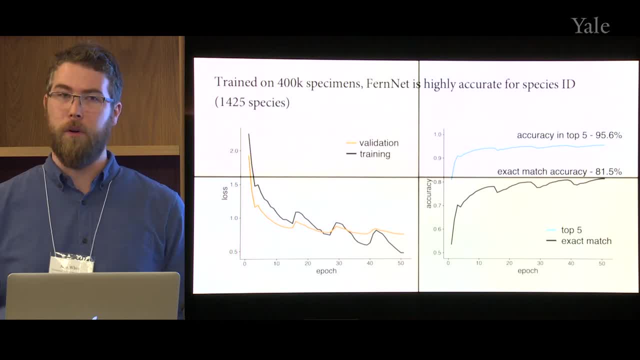 And we talked a little bit this morning about epochs, Which are individual periods where you cycle your entire training data set through the model, And so the model is constantly changing. What we're doing is essentially feeding images through this model. It has some prediction at the end. 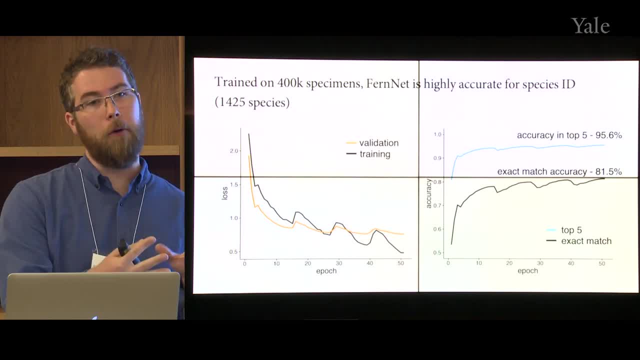 And there's an error with that prediction And we want to modify the parameters in a way that would reduce that error. So that error is the loss that you're seeing here on the y-axis on this panel. We want that loss to be plummeting as we are training the model. 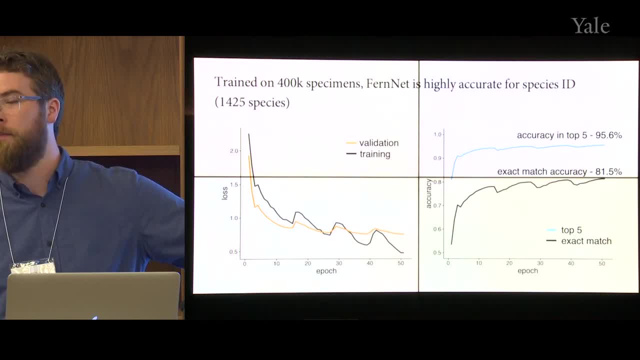 And there's a loss both based on the training data set and on the validation training set Or on the validation set, And usually what you end up with is That the training set has a lower loss Because it's starting to kind of converge on specific things that it's learning about, those images. 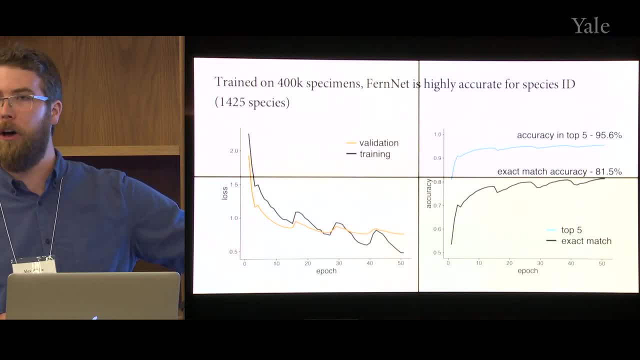 So as soon as that starts to kind of plateau, You stop training. But we also have accuracy. The accuracy is both the exact match accuracy, But also the accuracy in the top five. So in this case I'm showing the exact match accuracy. 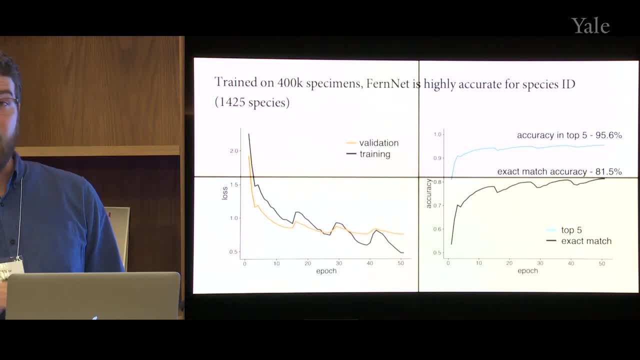 Which is about 81.5% for species. But for the top five predictions It gets the right species in that top five About 95.6% of the time And that is pretty incredible. Essentially, a lot of species are just differentiated by genetic markers. 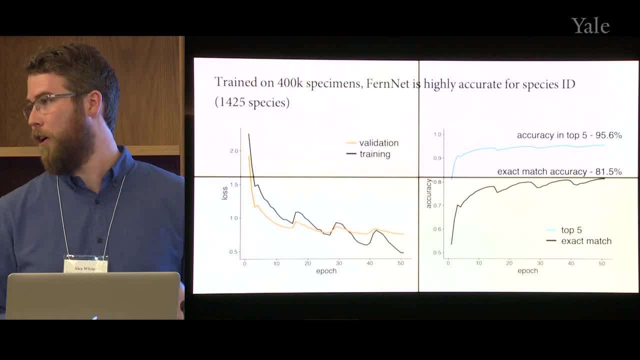 So the actual shape differences that the images are going to be able to pick up on Are almost non-existent, And so for the model to get that level of accuracy, I think is a forgivable level of error. So what is this FernNet using? 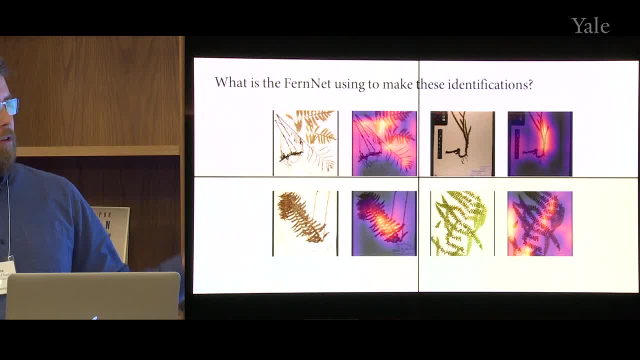 To make its identifications. Here I'm showing you four example images That were passed through the network And then four activation maps. Essentially, these are the pixels That the neural net found most interesting And most relevant To making a prediction. 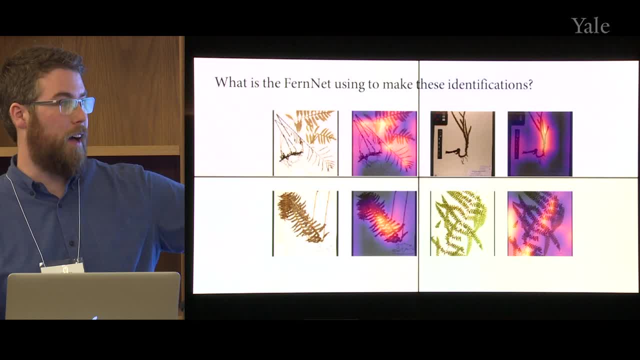 And the good thing is that the heat Or the hot colors in these heat maps Are over top of the plant And not on the label. It's not learning how to read the label. It's learning something about the images. We can also make some really cool things called feature maps. 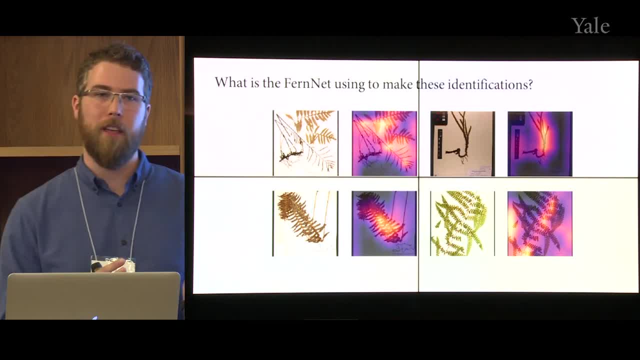 Essentially, what I'm going to show you next Is the different output of specific layers in our neural network And essentially what we would be looking at Is what the filter might look like That would activate, for that layer of the model, Earlier layers in these image recognition models. 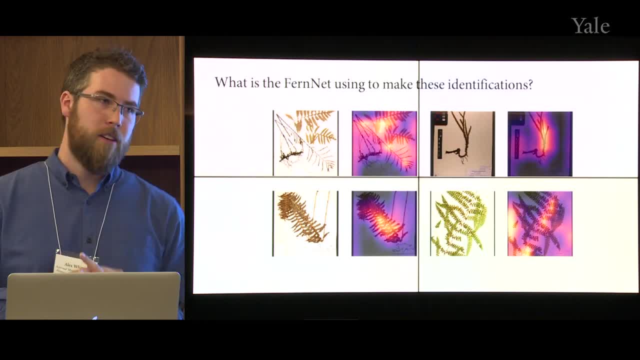 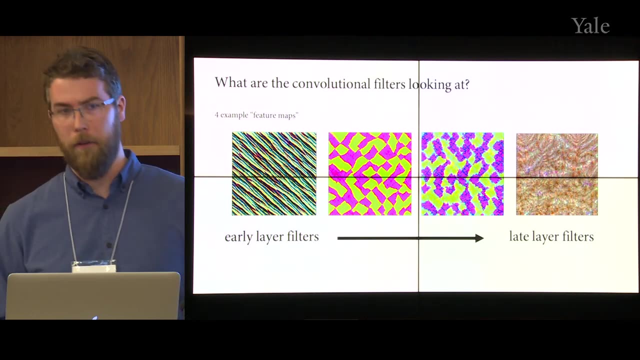 Tend to look more like shapes and patterns, And high level layers tend to be Kind of very specific for making those final distinctions Between, say, species A or species B. So here are four example feature maps. There are hundreds of layers in this model. 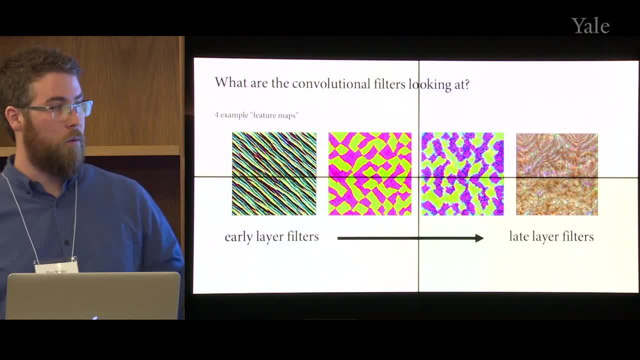 So I can't show you all of the feature maps. But what? How they built these Is by randomly populating an image with colors And then optimizing that image So that it would maximally activate that layer. So, yes, they look technicolored. 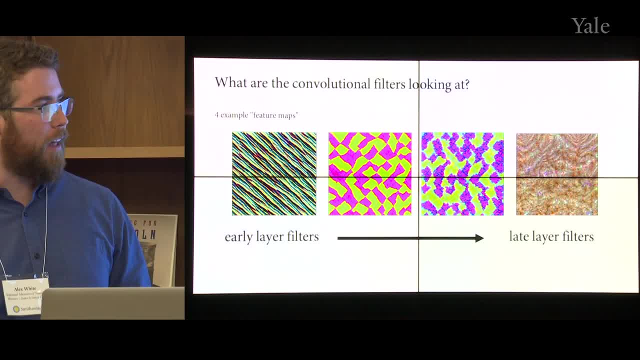 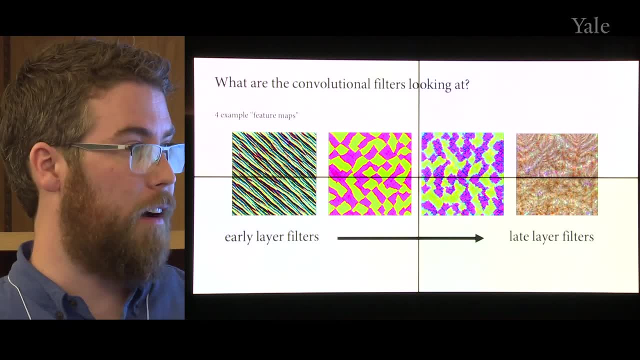 And more like the 90s color palette of neon. But the colors don't matter very much, And that's, I think, a really important part about our model Is that it's not activating by color. The colors tend to be very invariant. 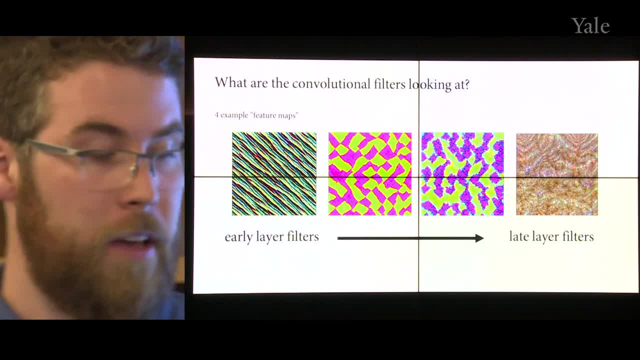 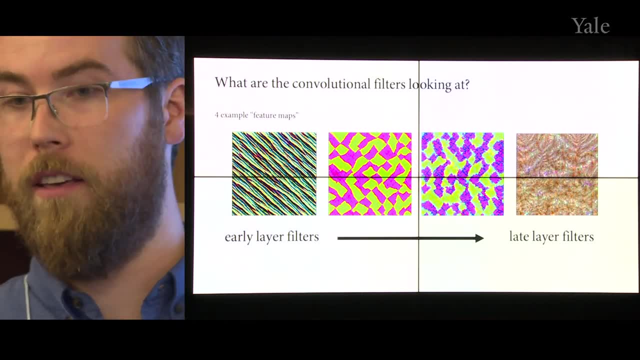 The shapes are highly variable And it's really more about shape. So you can see that later filter Maybe if you squint your eyes. It looks a little bit like a complex fern frond, So it's kind of getting towards our fern shapes. 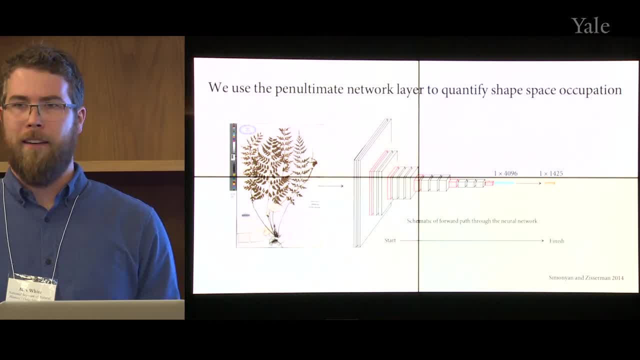 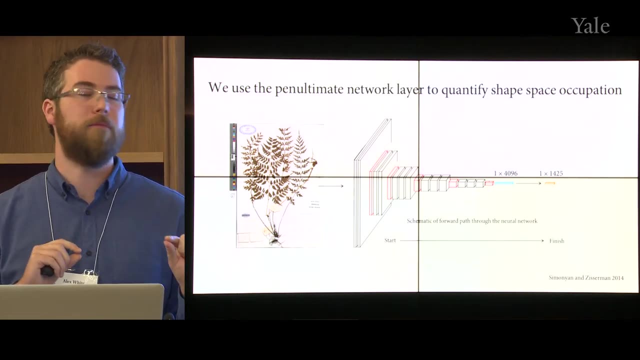 Okay, we saw a little bit about Why or how these models work To generate from a very complex data input A very low dimensional or single two dimensional Vector At the very end, And that vector, The 1 by 496 vector. 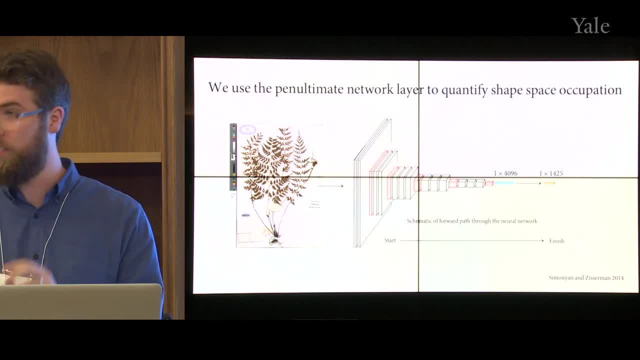 Right before it gets to the 1 by 1425 vector, Which is actually the probability That our image is within the 1425 different levels. That 496 vector is the one that we want to project In our UMAP space. 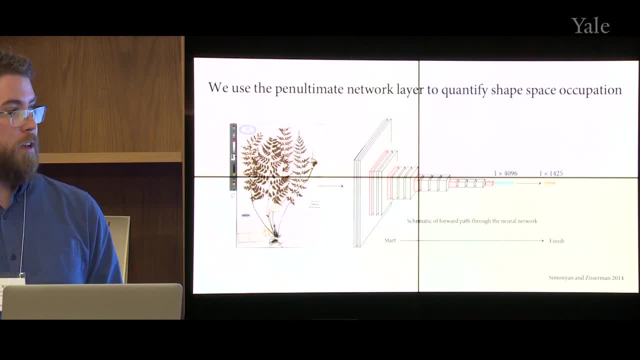 Like we saw earlier today with the Pixplot projections, In this case we're using a model That was specifically trained To understand the differences of species shapes For ferns, So we're not using the larger Kind of front end model. 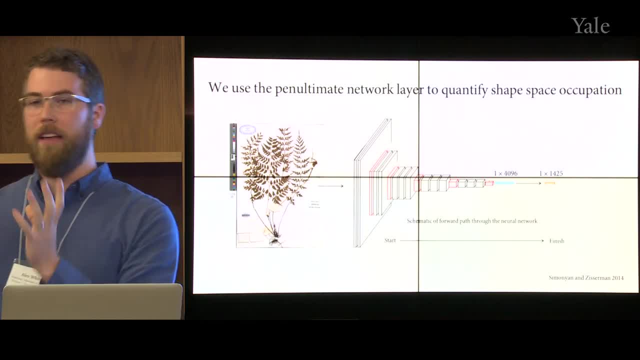 From ImageNet or ResNet Or something like that. That's pre-trained. We're using a model that's trained on these things, So we think those feature embeddings at 496 vector Is actually a really useful vector, Not for trying to understand the variation. 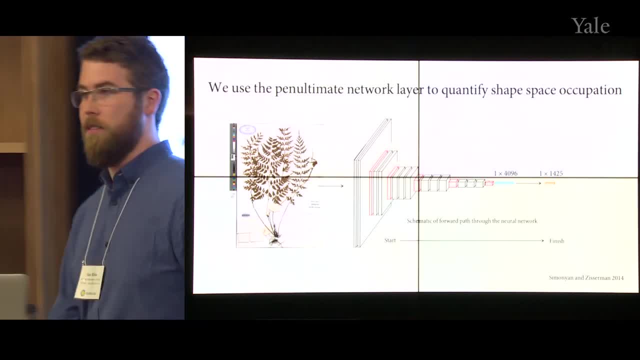 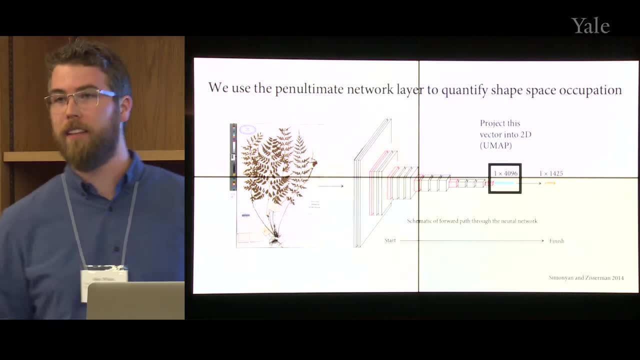 And say the label or this color ramp, Because every one of these images has that. So the model should have basically Kind of stopped learning about those. So we take those And we project them into a two-dimensional space And we can get our shape space. 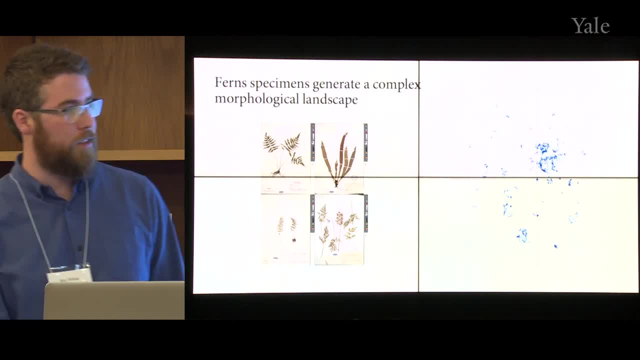 For ferns. So in this case, what we're looking at Is a two-dimensional projection Of each point is representative of one of those images. Just like we saw earlier today With the cool visualizations that Pixplot generated, We could look at this image. 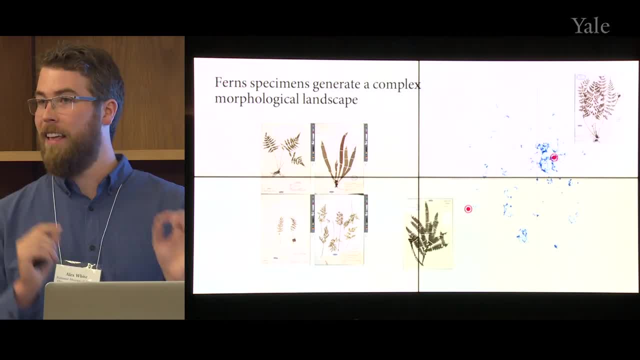 And kind of drill in And look at each individual specimen And where it's positioned Within this shape space. So here I've just thrown up two example images And we see that they look quite different from one another. There is actually a Euclidean distance. 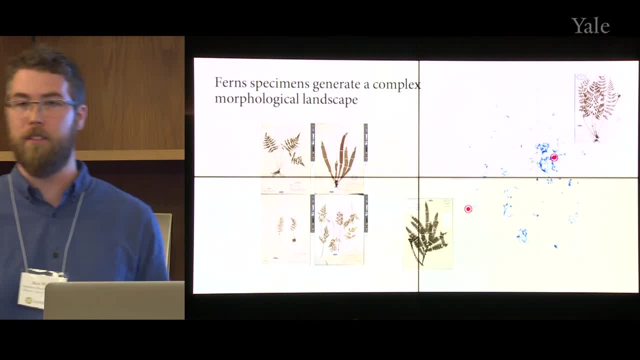 That is preserved in this projection, So we can measure the distance between them As some aspect of their shape, dissimilarity Or similarity, And we can then use that To understand this latitudinal diversity gradient. So here I'm actually now just dividing the world. 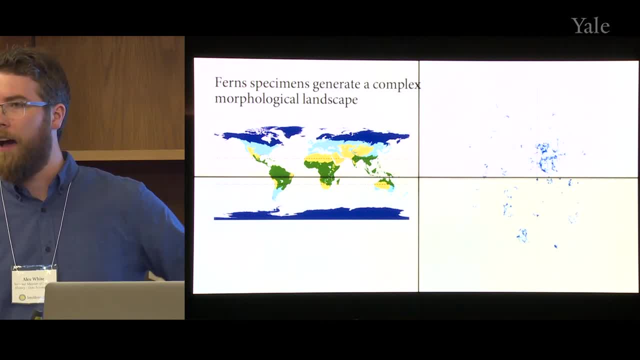 Instead of looking at latitudinal differences continuously, I've just divided the world into four unique kind of groupings: Tropical climates, Mountain, desert climates, Temperate climates, Which are the blue ones, And the dark blue is the polar climates. And now I'm just going to label our shape space.